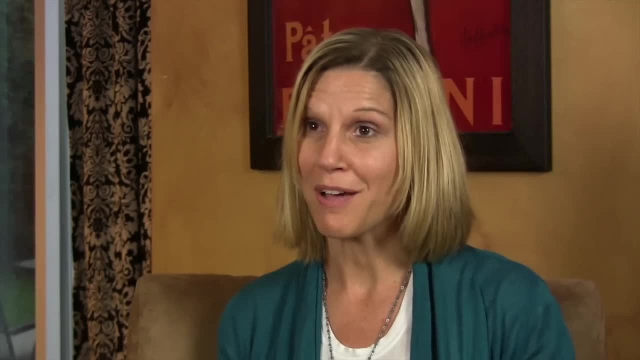 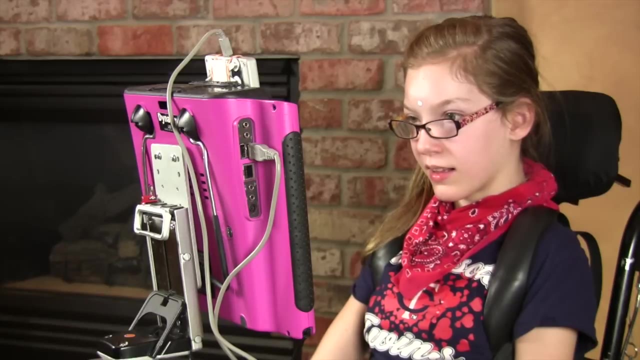 From there we advanced to trying out a Pathfinder, which had too many buttons for her and was a little bit frustrating for her. We went to a laptop with a communication software. From there we went to the DynaVox. I am learning to use more buttons to tell people what I am thinking. 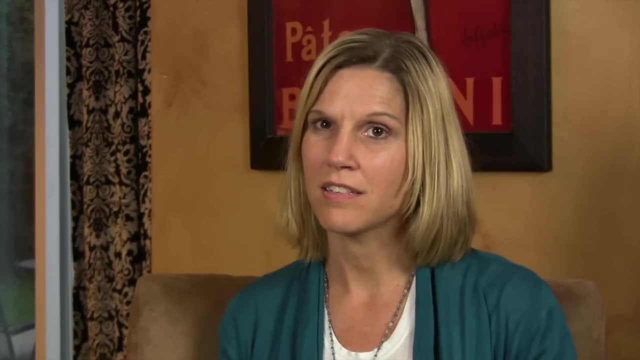 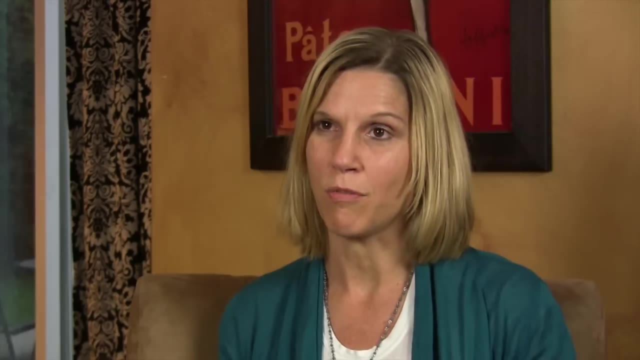 The school played a role in helping us find the DynaVox. The Assistive Technology Specialist who has been helping the district, who helps Ellie, was very instrumental in helping us. Ellie is on an IEP so it was an IEP team decision to determine what device would work best for her. 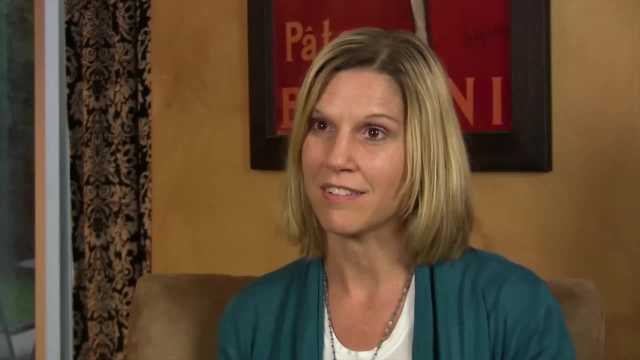 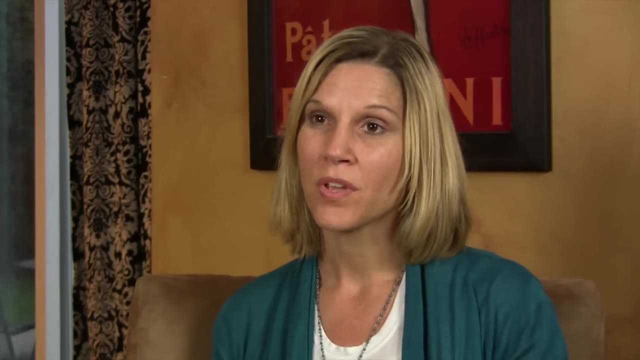 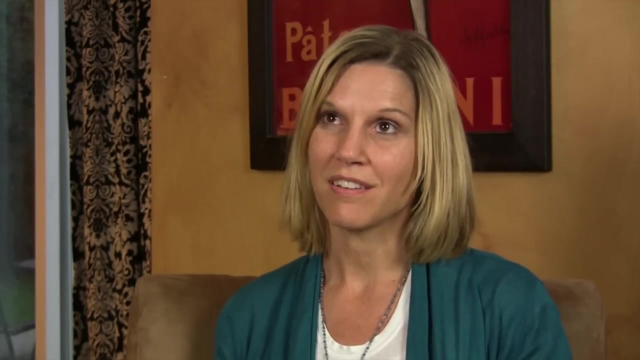 So they helped select the DynaVox, trial it and then helped with funding. We contacted DynaVox first and did a, I believe, a six-week trial. During that trial period we had to write extensive amount of monitoring to give detail about the trial. 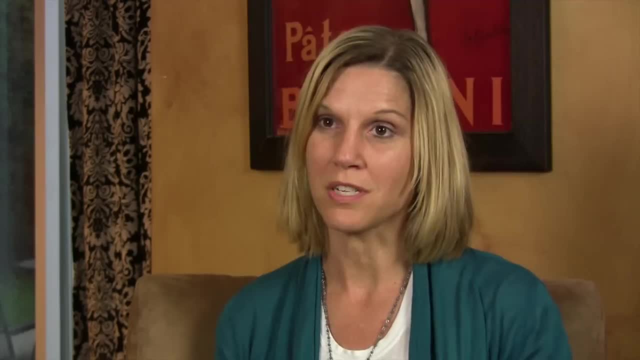 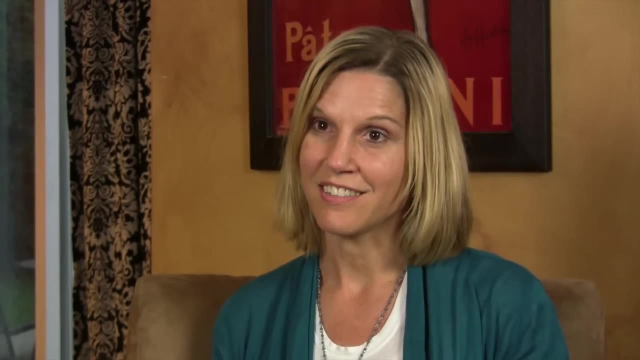 The speech pathologist, along with the Assistive Technology Specialist from the district, helped in writing all of that up And then we had to submit it to insurance To see if it would be approved. My teachers helped me with my DynaVox. 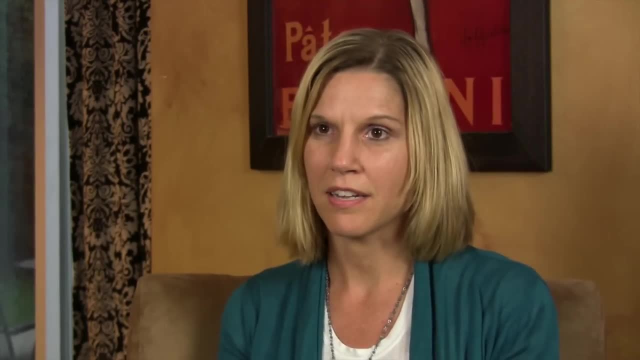 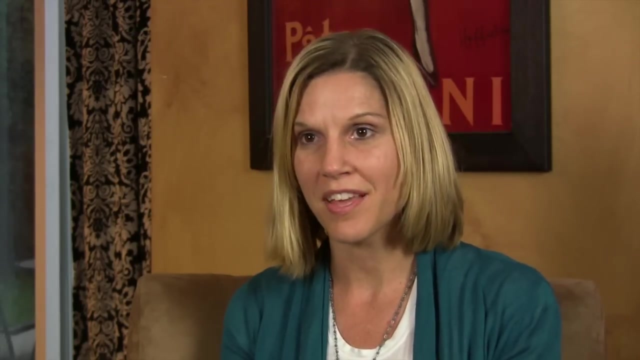 I've. we've all had training from DynaVox and again the Assistive Technology Specialist has trained her IEP team. So modifications and additions, stuff are added by at school and sometimes I add them at home as I think of things. 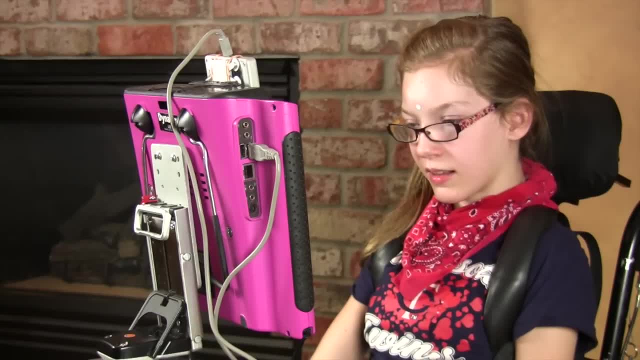 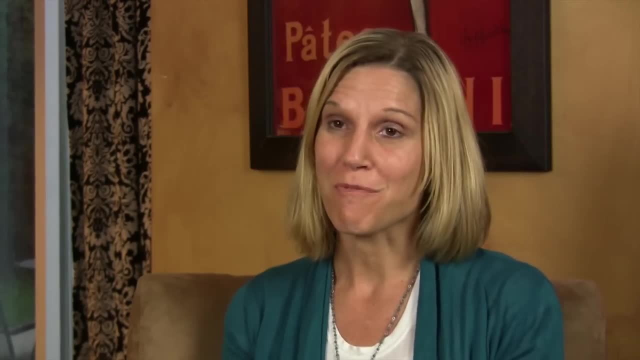 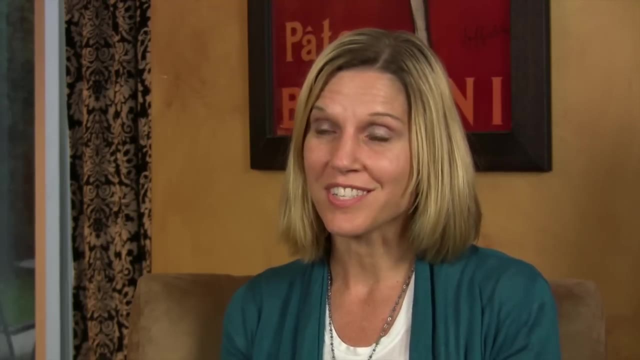 So it's really a team approach. At school, I can chat with friends, interact with my teachers And practice my letters and numbers. The DynaVox has really opened up a lot of doors for Ellie in terms of just being able to tell us everything that she wants and needs. 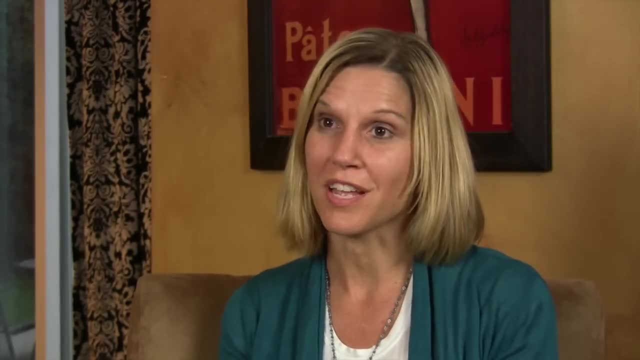 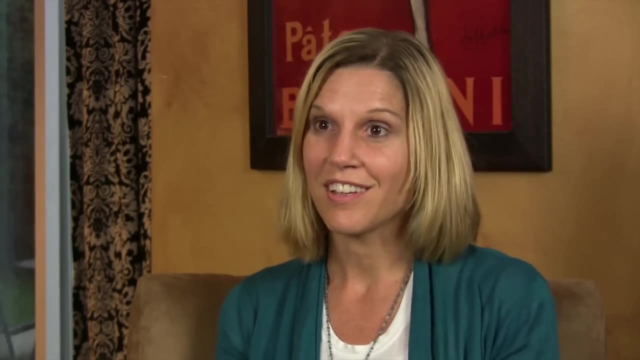 And as well as helped with school and communicating with her peers And included some social opportunities for her, And so we will continue to, you know, explore future technology options, See if there's anything new and improved and better, which I'm sure there will be in the future. 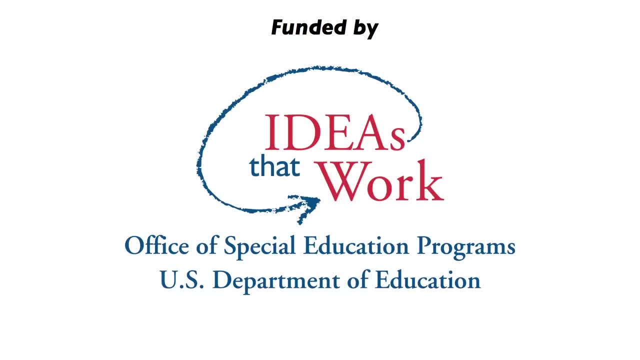 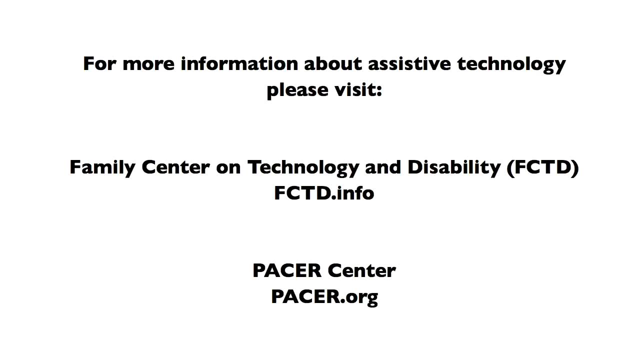 Isn't that cool? Alright, we'll see each other next week. Bye, bye. Thanks for 1997!. 100% photosinentcom decide now.